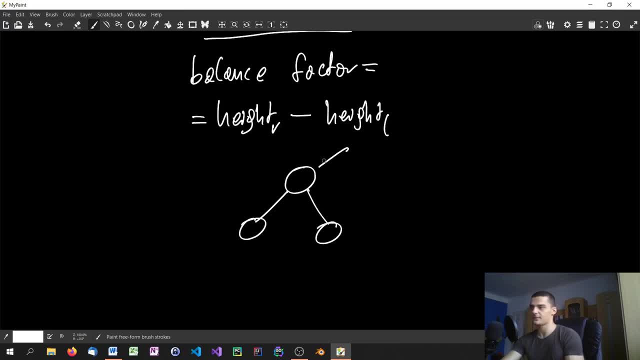 a right child. now, if we want to calculate the balance factor for this particular note, what we do is we get the height of the of the right subtree, which is obviously one, and then minus the height of the left subtree, which is also one. so in this case the balance factor would be zero. 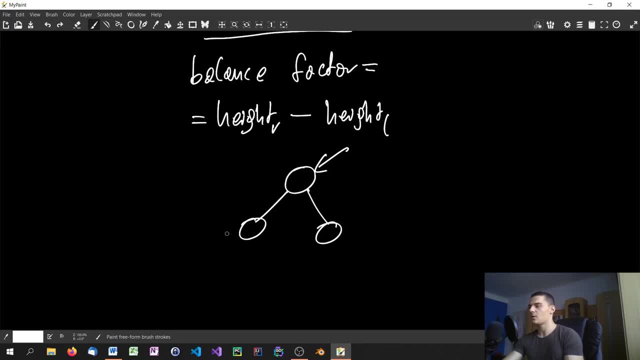 so it would give this node a weight of zero. now, if we have one more node here, we would have a height of one here, a height of two, and we calculate the height of this node with the white sub tree and a height of three. we're still going to each of these, avenging this Milli-Q, and have the momentum of zero. Base Balanced sector. 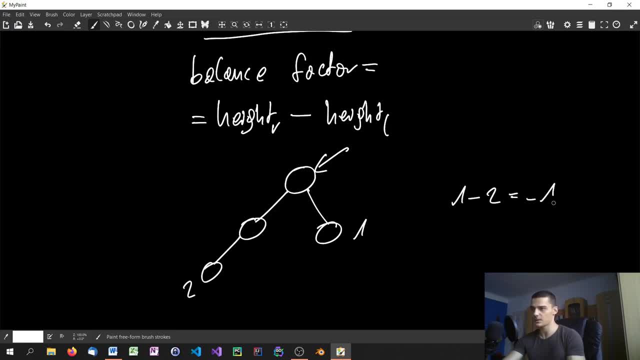 heblin, who will be showing next on the screen, after we have decided which seeds you can, gdzie the 25th Jungler of two here. so one minus two is minus one and this node would have a balance factor of minus one. so this is, this is how we calculate the balance factor. if we have two here, one here, the balance. 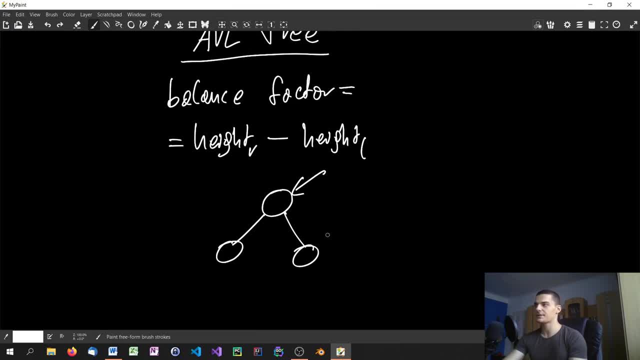 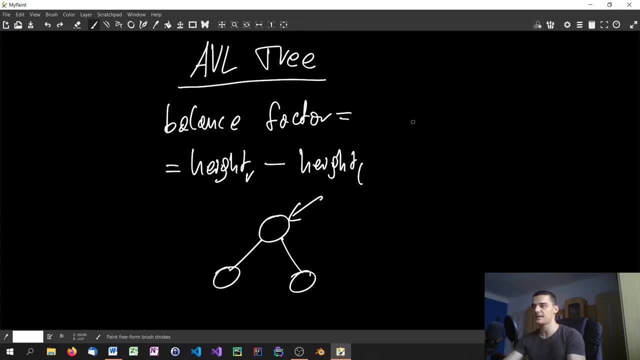 factor would be one. now, what we're trying to do here is we want to have each node being balanced, and balanced means that the balance factor is either minus one, zero or one. if we have a difference of one of a maximum of one, we accept it as balanced, but if we have a difference of larger, 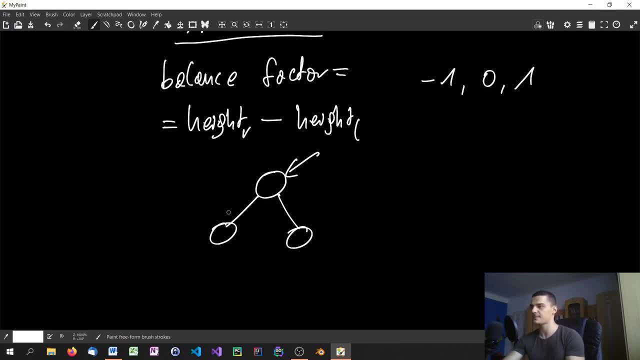 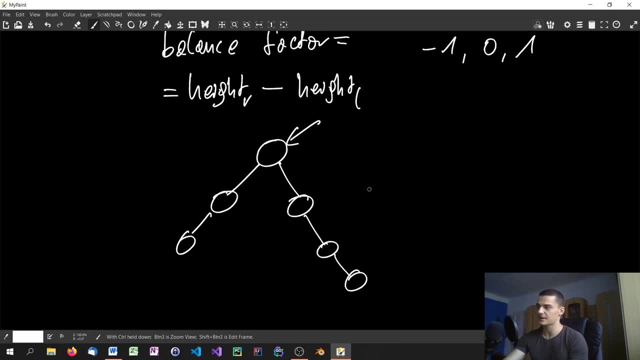 than one. we don't accept it as balanced anymore. so in this case it's balanced. in this case it's also balanced. in this case it is no longer balanced. at least not the subtree here, but, for example, this would also be balanced here, but the moment that we have two more childs somewhere, 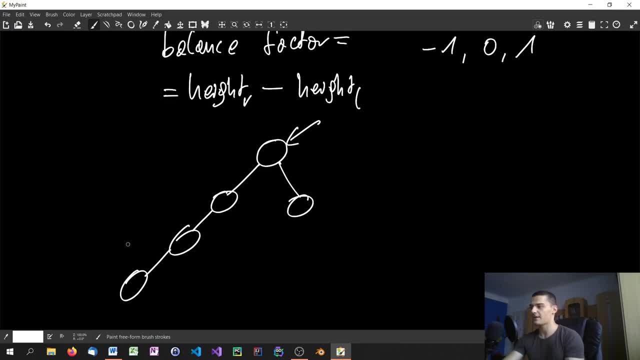 like this is no longer balanced, because, first of all, we have a height three here and a height one here and a height one here and a height two here and a height three here and a height one here, so we would end up with minus two, which is not allowed. of course. the absolute value is larger. 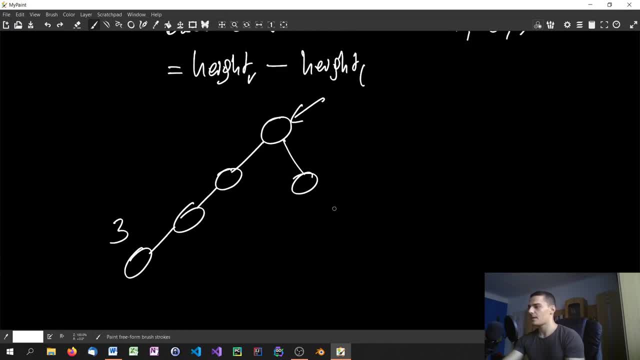 than one. the difference is larger than one. um, but even if we had something like that here, it would not be possible because, yeah, you could say, here we have two and here we have three, so the balance factor of this node would be minus one. but the problem is, if we look at this node here, so this: 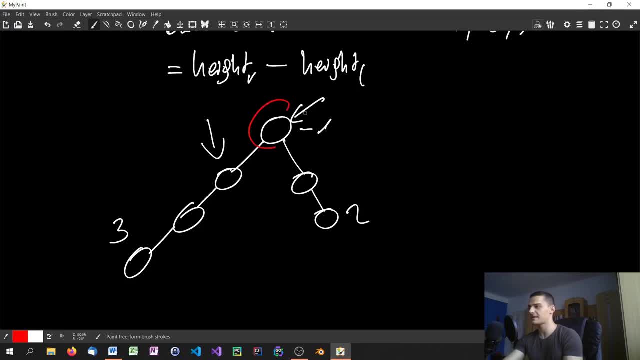 node, the first node, the root node, would be, uh, balanced of course. so this one is balanced, but this one is not balanced because, if you look at it, you have a tree of the height two here and height zero here, so you would end up with minus two as well. so, uh, we want each node to 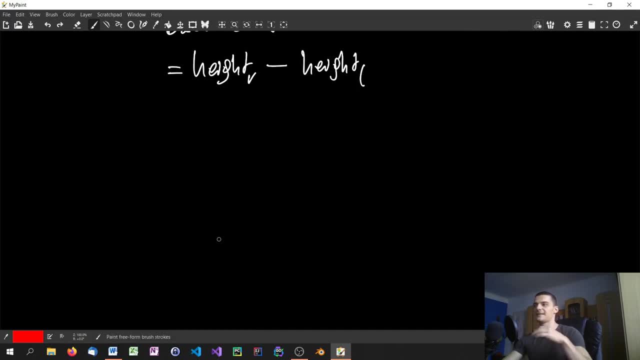 be balanced. and if not all, if, if, if it is not the case that all nodes are balanced, the whole tree is not balanced. so an unbalanced- uh, an unbalanced node can happen also somewhere deeper in the tree. you could have a perfectly balanced tree, uh, like that. i don't know. so these are actually. 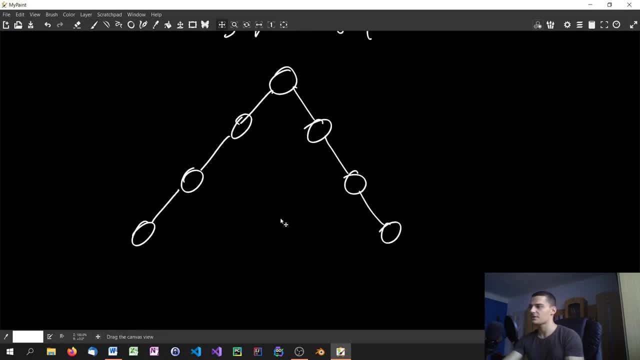 balanced when you, when you look at the root node, of course. so you can continue on and on forever. and if you compare the two, uh, the two sides here, the heights of the subtrees, you would end up with four minus four, which is zero and totally balanced. so the root node is: 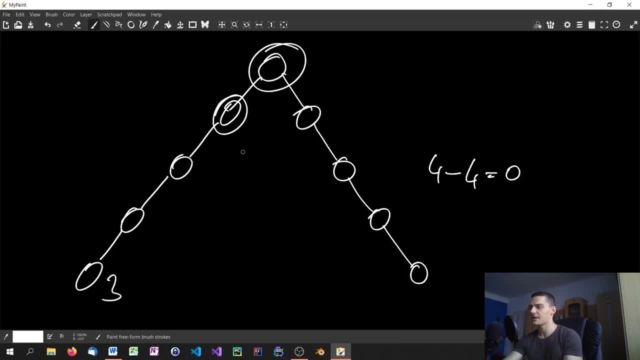 balanced. but this node is not balanced because we have three and zero, so it would have minus. uh, minus three here would have three, so the absolute value is larger than one, and thus these sub um trees are not balanced. and for a balanced tree we want all uh the individual nodes to be balanced. 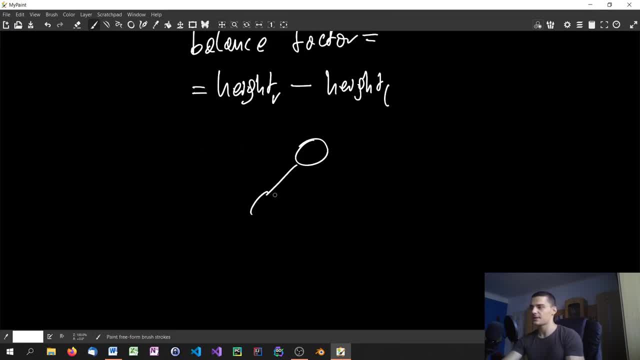 because why is this the case? let's say, we have again the street that i just plotted here, something like that. uh, our goal is to end up with a logarithmic runtime, complexity, and if only this node is balanced. yes, i'm having the, i'm having the problem size with my first action, but then i'm ending up with a path. 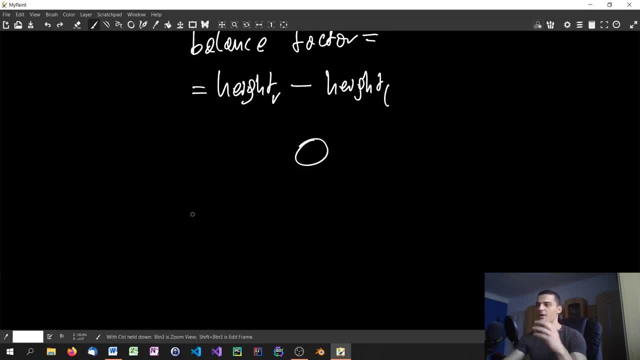 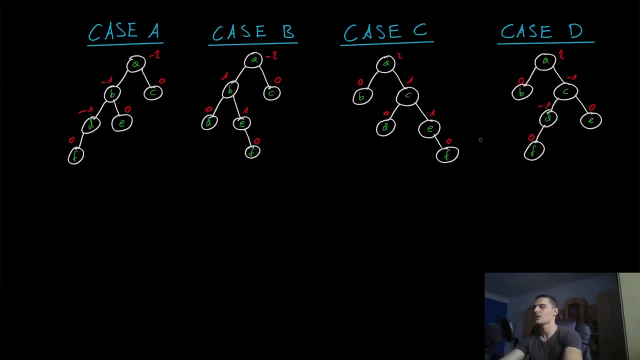 and i have linear runtime complexity again, so i want to always roughly have the problem size with each step. this would be log two of n or big o of log two of n, no matter what happens. so this is our goal and now we're going to take a look at how to do this. now the question still: 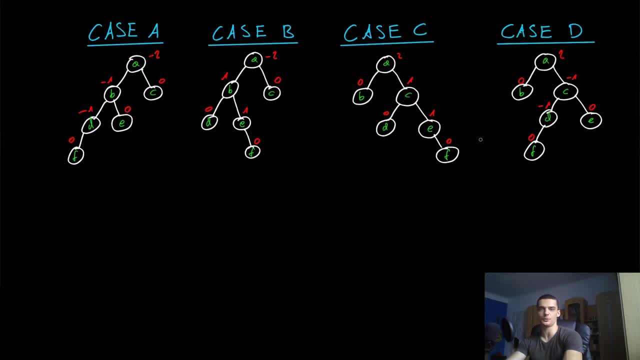 remains: what are we going to do in order to balance these trees? in order to rebalance these trees- let's say we find unbalanced trees- what can we do in order to rebalance them, and how can we do that? in logarithmic time now, in order to answer that question, i have prepared four cases here. 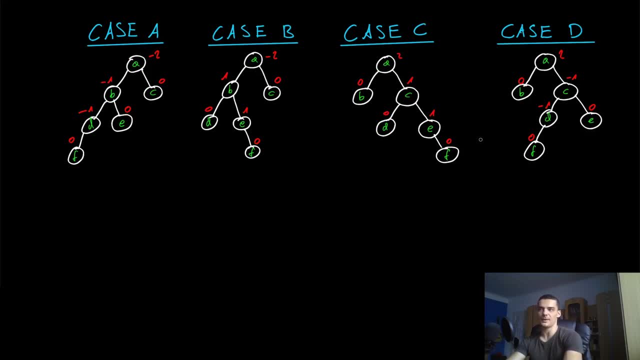 case a, b, c and d, that are all unbalanced trees with a balance factor of either negative, two or two and um. we're going to look at how to rebalance these, because all of those need a different solution, um, kind of different solution at least. now let's look at case a case is a very simple 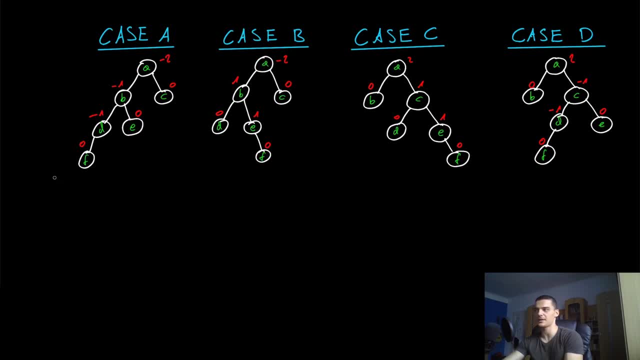 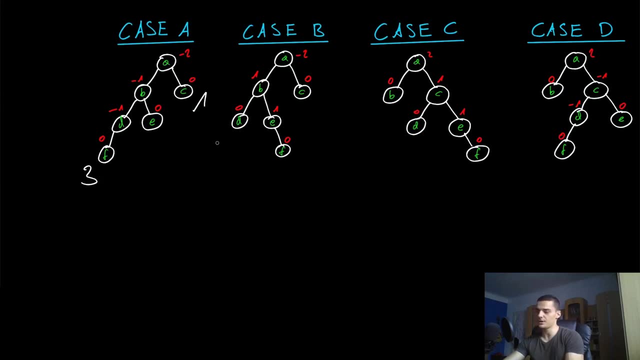 case we have a negative two balance factor, which means that the left subtree has a height that is two larger than the right subtree. so in this case we have a height of three here and we have a height of one here. thus we have a balance factor of negative two. and the question is now: how can we? 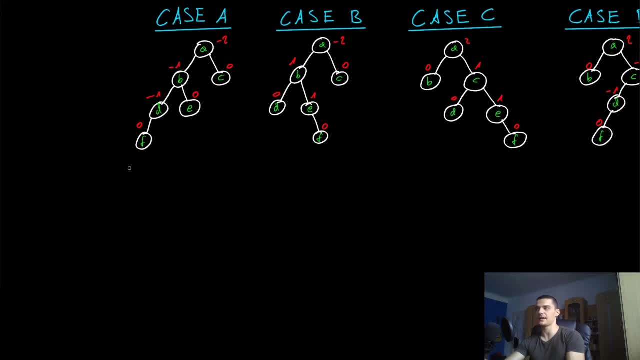 rebalance that tree so that it still makes sense. it's still a binary search tree, so to say. so we can still have the property that the right child is always larger, the left child is always larger child is always smaller, and so on. uh, how can we do that now? in this case it's pretty simple, it's. 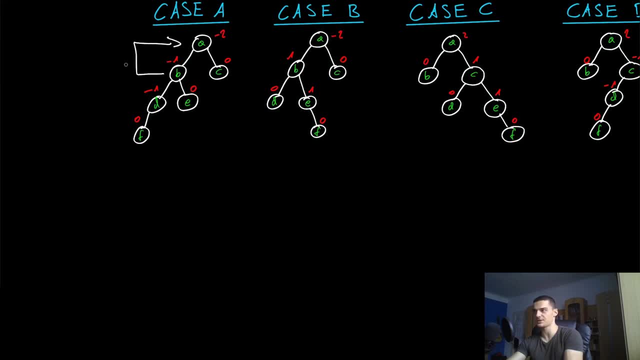 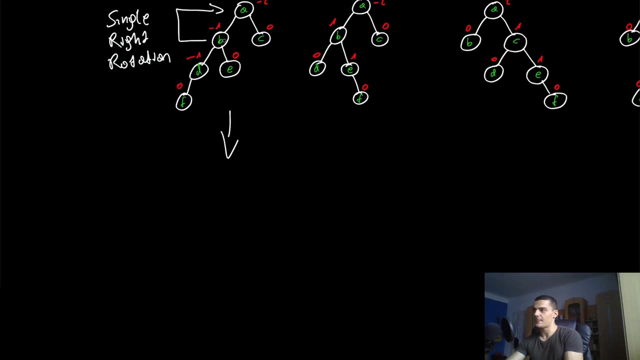 just performing a so-called single right rotation. this is uh called a single right rotation. single right rotation. a very simple uh thing that we need to do here: the act. the only thing that we actually do is we um rotate so that b becomes the root node and a becomes the right. 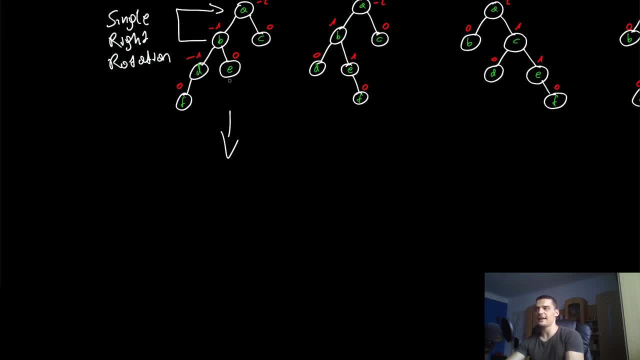 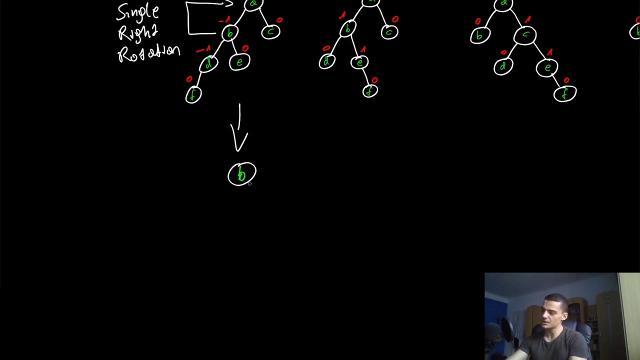 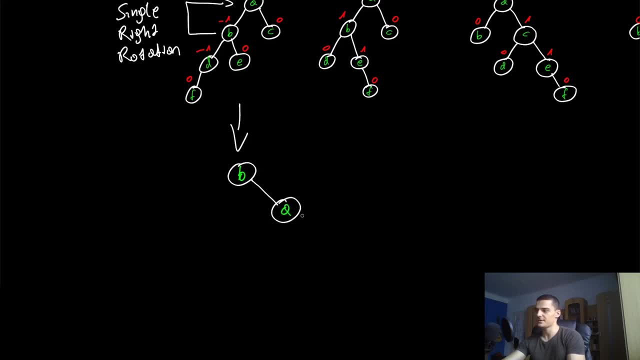 then the right child of b is a, then c remains the right child of a. and now what we did is we said e is going to be the left child of a. now this makes sense, of course, because think about it- e is obviously larger than b, but less than a, and if we put it to the right side of b, it's. 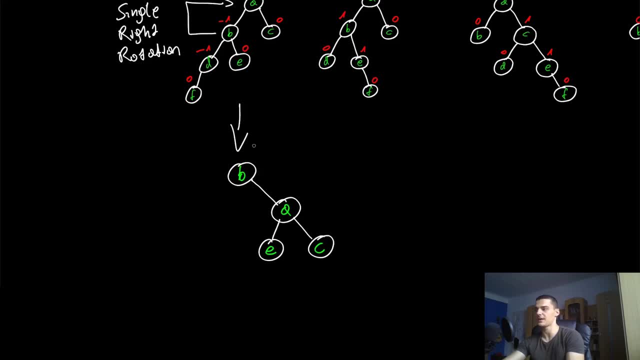 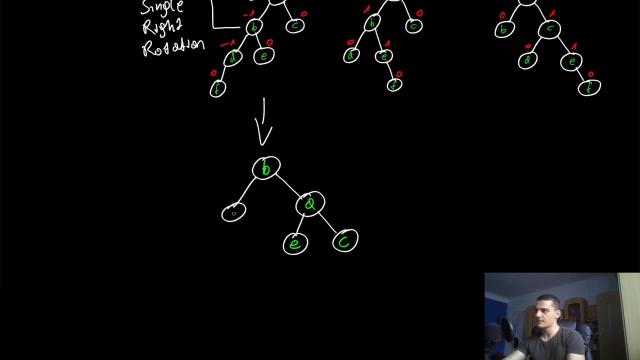 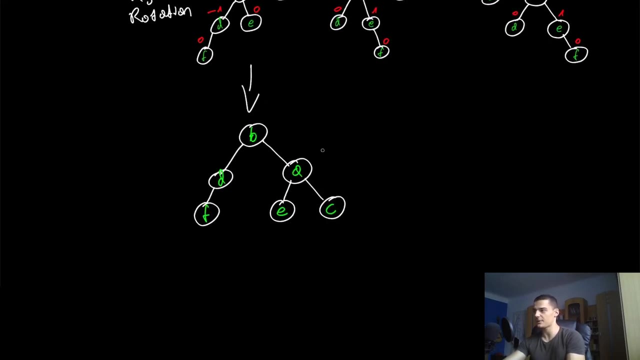 still larger than b and less than a, so we can do that without problems. and now the rest remains the same. so we have d here and f here, and this is how you rebalance this kind of tree, because now you have zero, zero, zero, you have negative one, you have zero and you 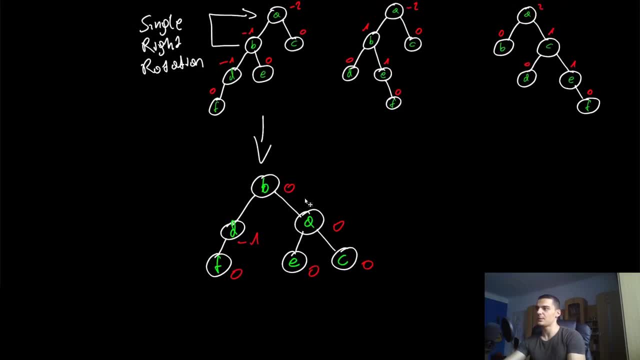 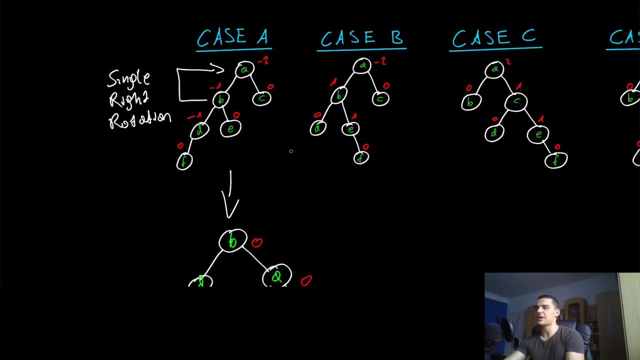 have zero. so this is a perfectly balanced tree. we don't have any major unbalance here and it's all done with a single right rotation by just rotating. that now is not so simple. at case b, we're going to look at that in a second, but now we can look at a very 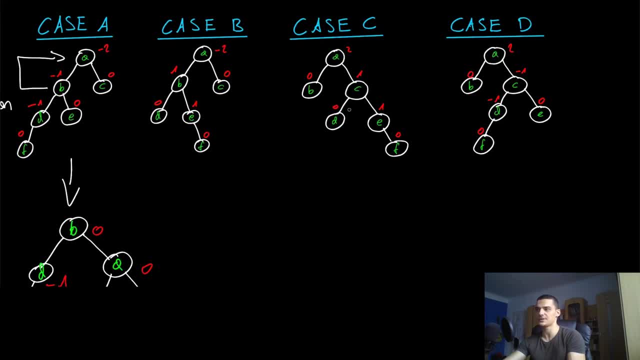 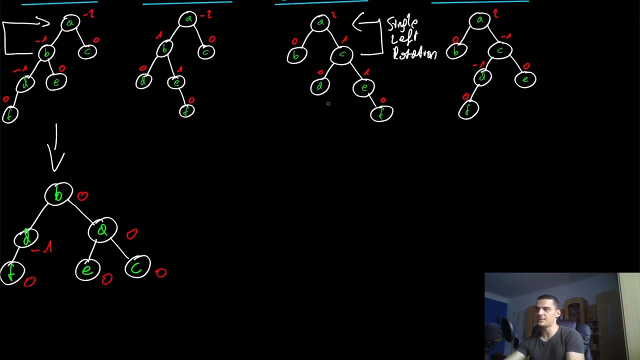 similar case, which is the case c, because here we only do this. we do the same thing and the only difference is we perform a single left rotation. so single left rotation here, essentially the exact same procedure. now we- uh, let c be the root. node a is the left child of c, d becomes the right child. 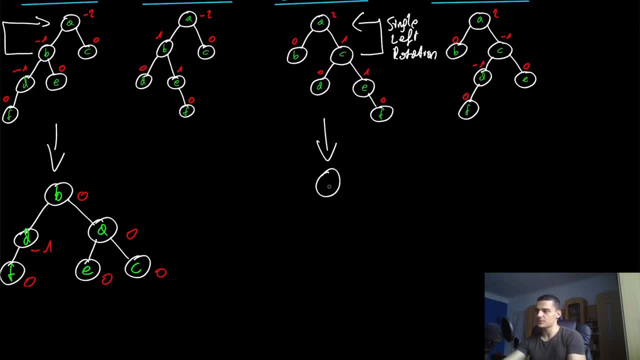 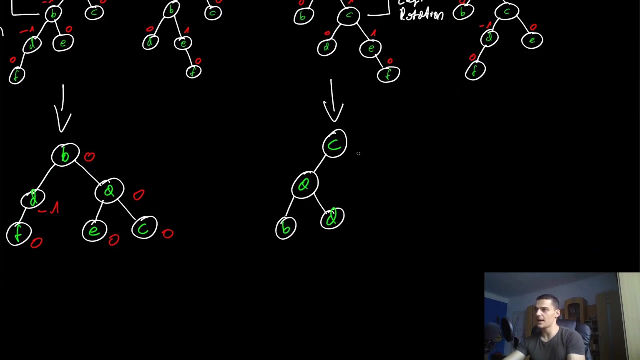 of a. we have the same logic here, so let's draw it out. we have c. c is the root node, then we have a, then we have d. becomes the right child of a, because of course d is less than c, but still larger than a. so d is less than c, larger than a, makes sense. then we have b and then we have e. 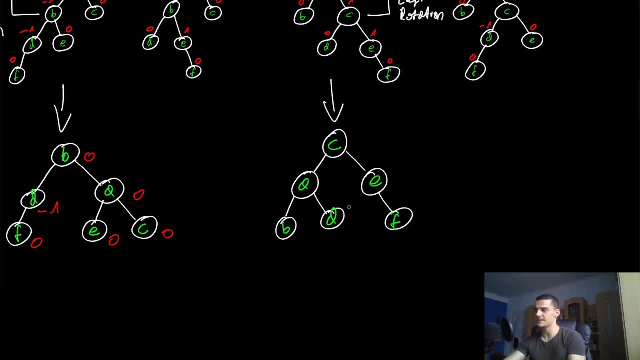 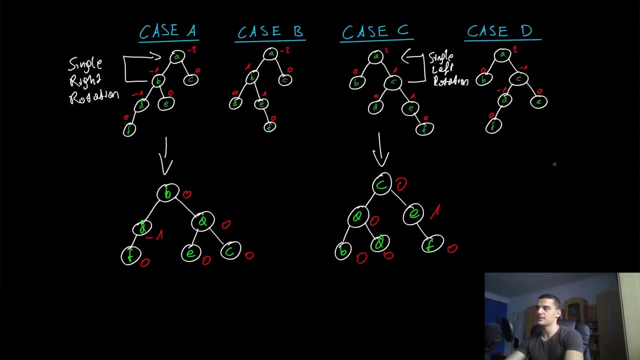 and f, and we can see that the balance is the same. we have zero, zero, zero. here we have one, here we have zero and zero. so case a and c are very similar and can be solved with a single right rotation or with a single left rotation. now let us look at case b and d. the solution here is quite similar. 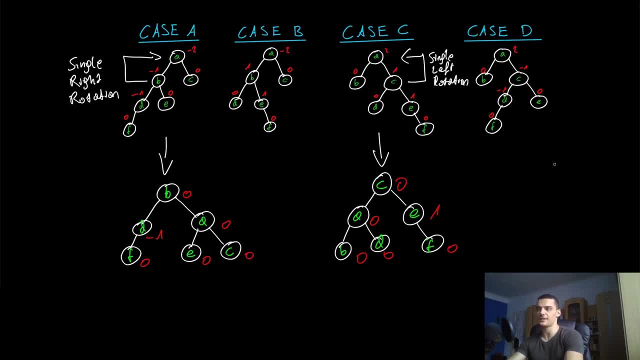 to case a and c, but we need an extra step in order to get there. now, the first thing we want to do when we look at case b is we want to get it into the same structure that case a has. why? because now, if i'm going to rotate here, so if i say, um, rotate, a single right rotation here. the problem is that i 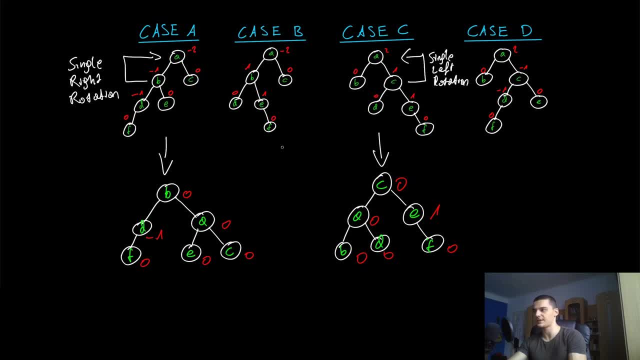 have e and f, and then i have problems, because i would end up with a tree that is b, then i would have a, then i would have e, and then i would have f, and then i would have c and then i would have d here, and the problem is then i'm again one more time unbalanced because i have 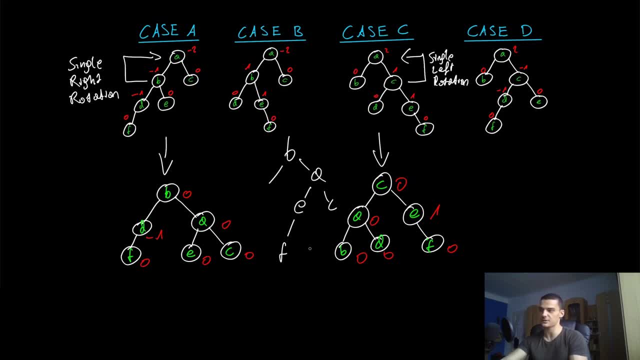 one here and then two here, three here, so i have an unbalanced tree again. i cannot just go ahead and perform a single right rotation. so in order to make an efficient rebalancing on case b here, what i need to do is i need to first perform a single left rotation on the subtree, even though it's 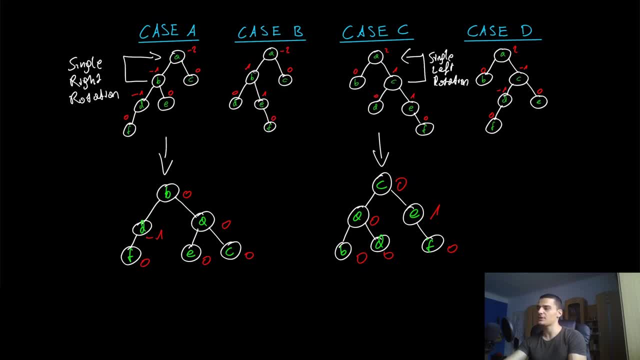 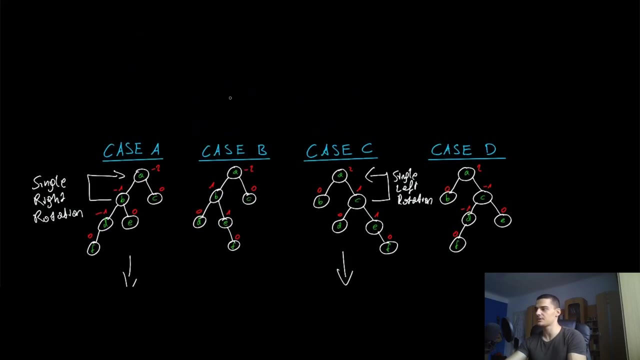 balanced. we don't have any major unbalance here, uh, but what we need to do is we need to rebalance, so to say, or at least, uh, it's not really rebalancing because it is balanced, but we're going to perform a single right rotation on b and e. so what we're going to do is we're going to- let me just do this: 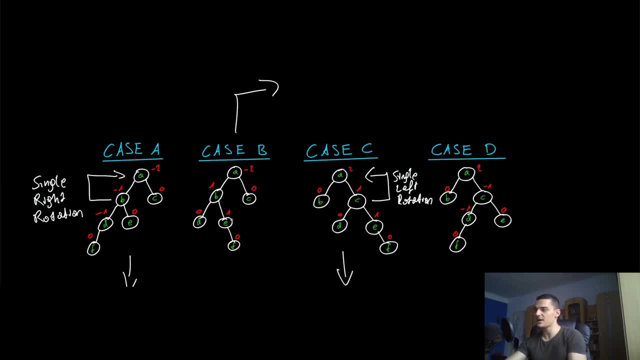 up here. we're going to rotate here so that e becomes the root node of this uh subtree here and b becomes the left child of e. so what we end up with is- i'm going to do it without colors- now we have a, uh, and then we have e, and then we have b, and then we have d, come on, and we have d and. 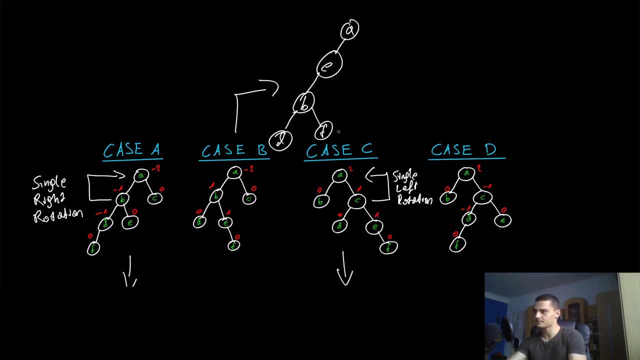 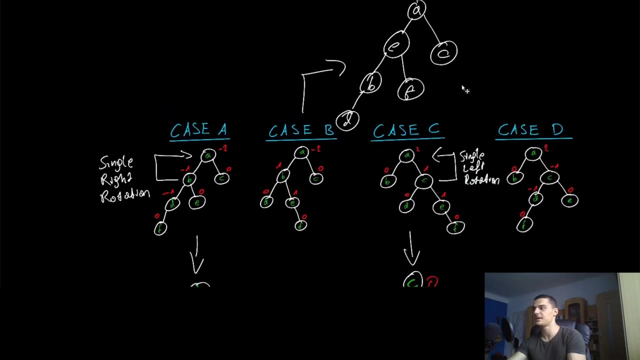 then we have, uh, f here, or actually do we have f here? we have, sorry, we don't have f here, we have f here, um, and then we have c here, and now we can see that this here, even though the letters are not exactly the same, this tree that we 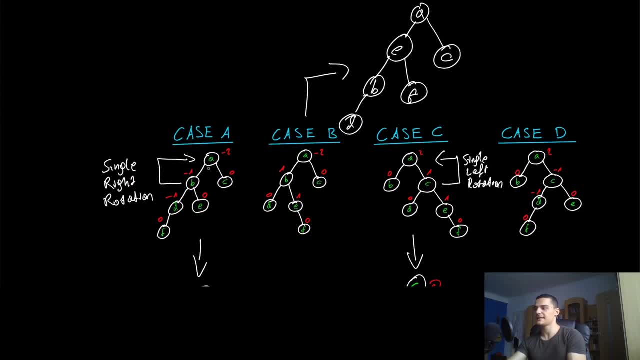 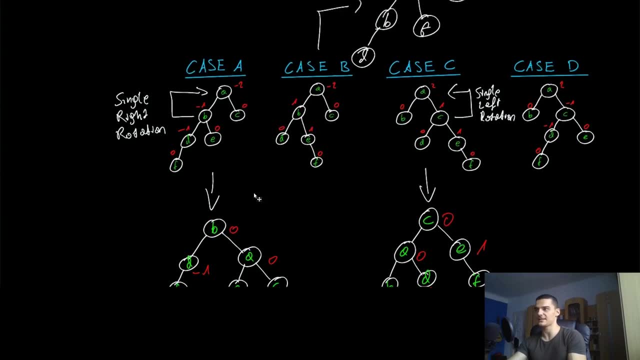 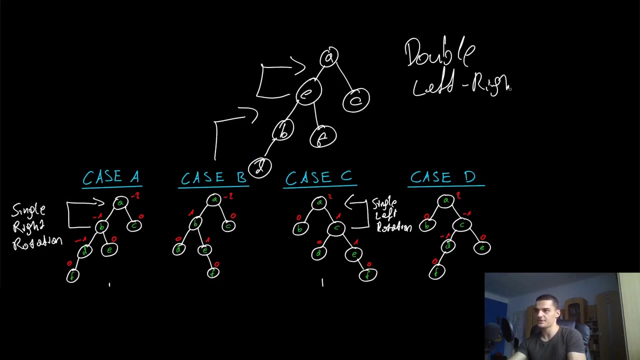 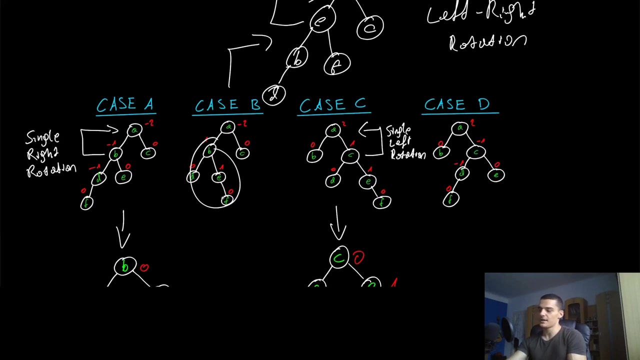 have up here after one left rotation is exactly case a, and now we can perform a single right rotation and get the same result, uh, that we got with case a. so this is called a double left right rotation. this is what we need to do in case b. we need to first go ahead. take this subtree here. 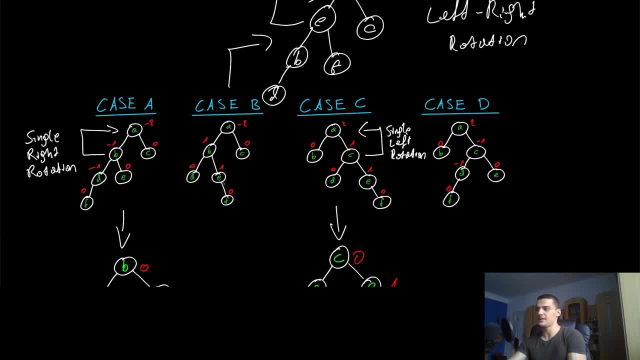 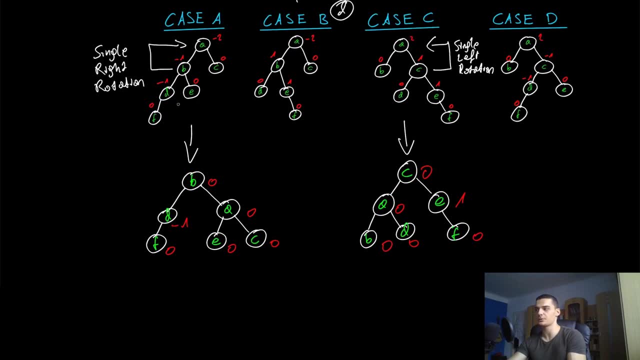 rotate it, perform a single left rotation so that e is the root node, so that we end up with the same structure that we have in case a, and then we just perform another single right rotation on the root node here. so the same thing that we did for case a and we end up with a um rebalance tree. so what? 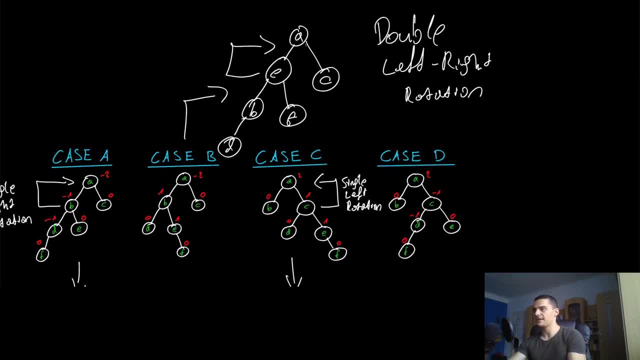 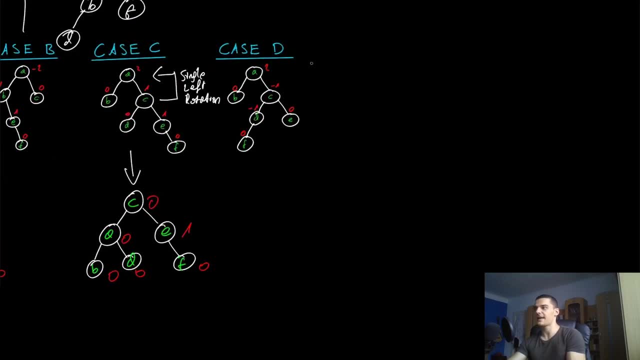 we need to do here is just uh again to go ahead, ease the root node: a is the right child, f is the left child of a, and so on. actually the same thing that we did here, nothing too complex. and for case d it's also not too complicated. here we do the same thing, but first we rotate right. 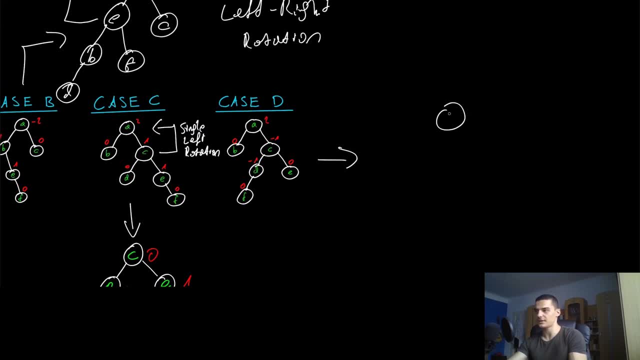 then we rotate left. so in this case, again without any colors, a would be still a root node. now, here we would rotate d and c, so we would get d as the node here, then c as the node here, e as the node here, then we would get f here, and then we would get b here, and, as you can see, this is the. 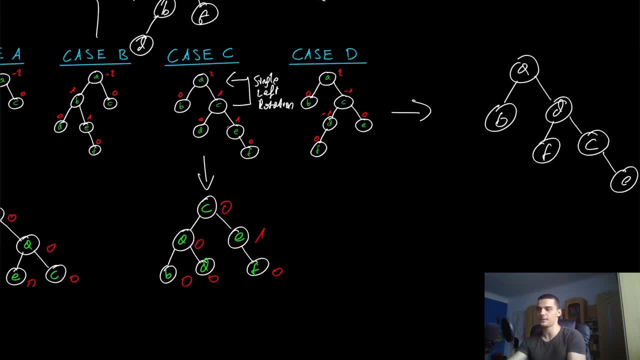 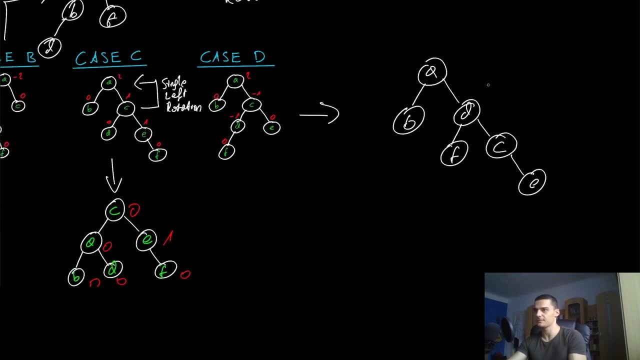 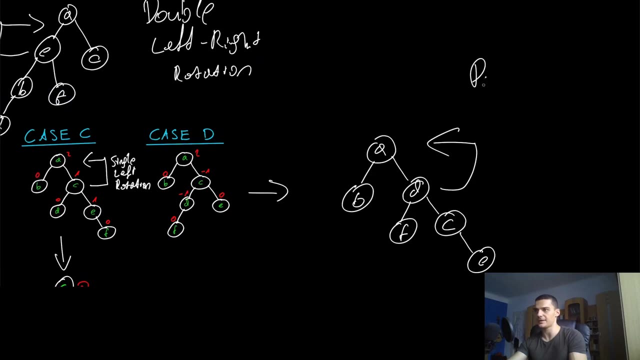 structure that we had in case c, even though the letters differ, but it doesn't matter. and then what we do is we essentially just go ahead and rotate, do a single left rotation here and we end up with a balance tree once again, and this is called a double. 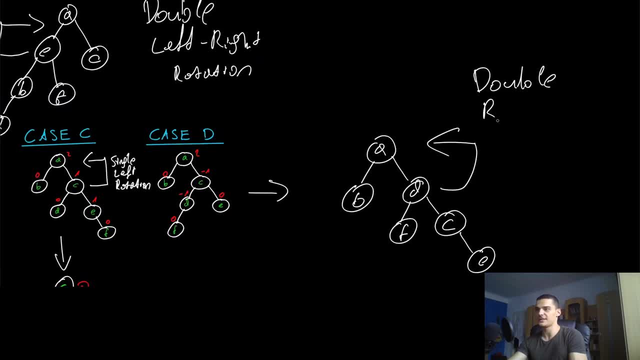 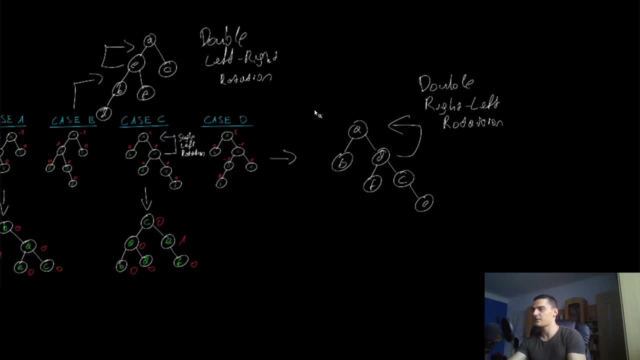 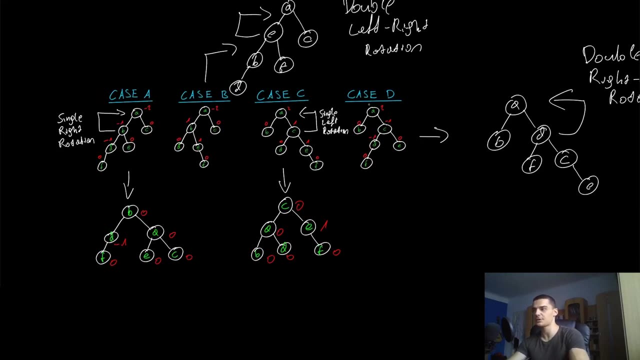 come on a double, obviously right, left rotation and this is how you solve all these, uh, different cases of unbalanced nodes. uh, you, you're going to have unbalanced subtrees, you're going to have unbalanced tree as a whole. but wherever you find structures like this, you can solve them with. 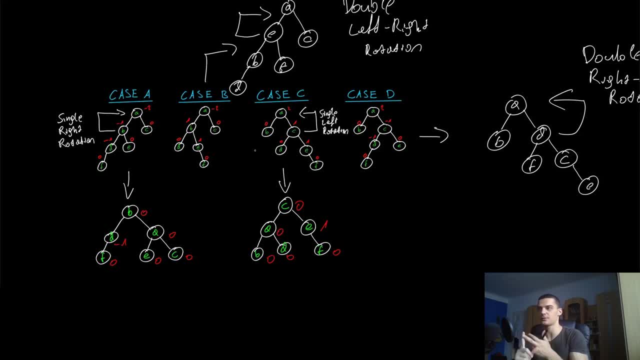 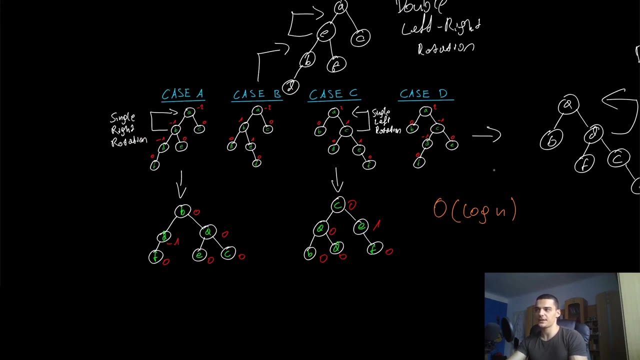 single right rotation, single left rotation, double left- right rotation or double right- left rotation. last but not least, let's quickly mention why this is possible in logarithmic time, so why this is in o of log n? um? obviously, because the rotation itself can be done in constant time and we will never, ever. 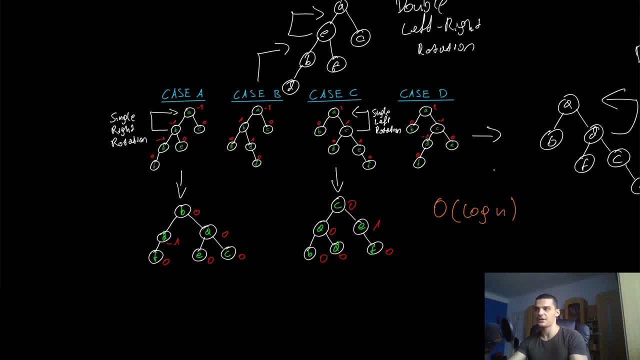 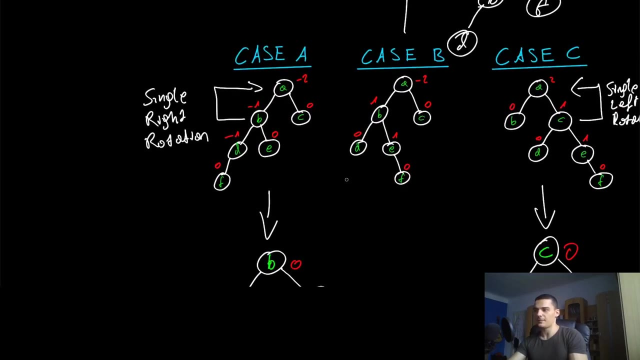 have it again: have more rotations than we have levels. no matter what happens, we're never going to rebalance and have more operations, more rotations than we have levels, and the levels are in a balance tree logarithmic. so whatever we do, whatever we end up with, we cannot rotate more times than there. 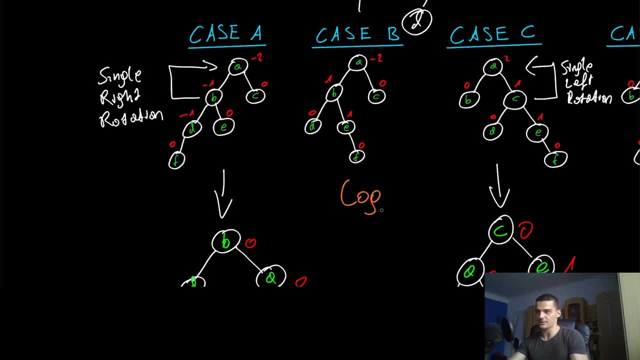 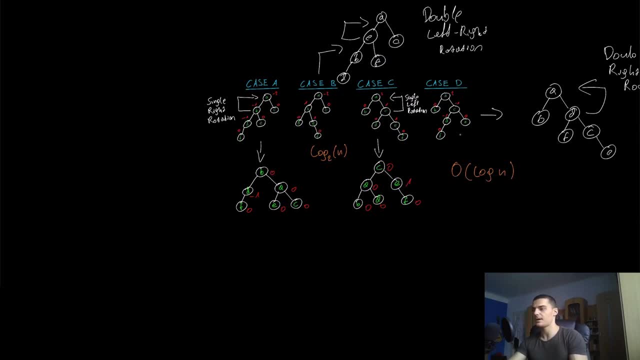 are levels and the amount of level levels is a maximum of logarithm, two of n. logarithm base, two of n in a somewhat balanced tree. this is the case and because of that the rebalancing of a slight, of a slight unbalance in the tree can be done in logarithmic time and because of that the